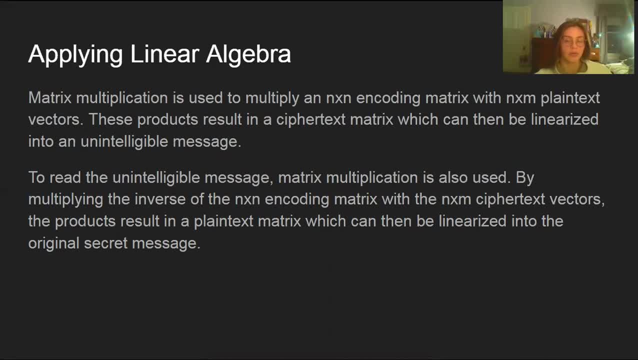 So with that, this is just a little overview about what we're going to do. So to encrypt our message, we will be using an encoding matrix and use matrix multiplication. We multiply the encoding matrix by the plain text matrix. This will result in a ciphertext matrix and we will 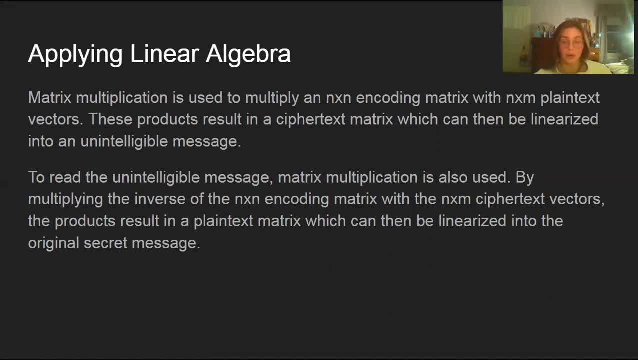 linearize this into an unintelligible message using code, And then to decrypt this message we will use matrix multiplication once more. We will instead use a decoding matrix, which is just the inverse of the encoding matrix, and we'll multiply that by the cipher matrix. 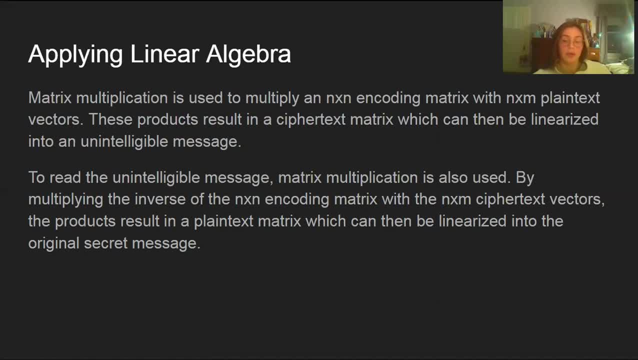 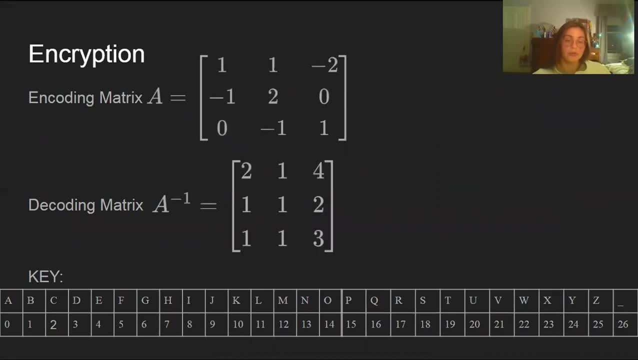 ciphertext matrix, which will give us the plain text matrix, which will then be linearized into the original secret message. So, to start off with the encryption, we'll need our encoding matrix, which has to be invertible, and this will give us the decoding matrix, And we'll also need to define a key. It can. 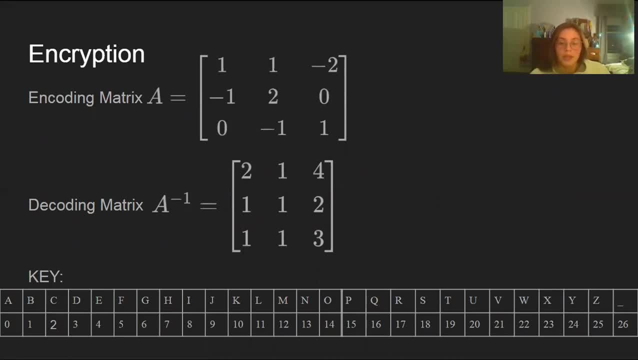 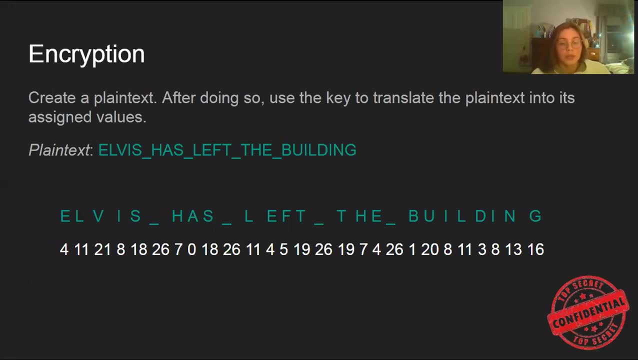 be anything you like. I chose the alphabet and a little underscore for my space. So now to encrypt our message, we need to start with our plain text message. I chose Elvis is in the building because I thought it was, or Elvis has left the building because 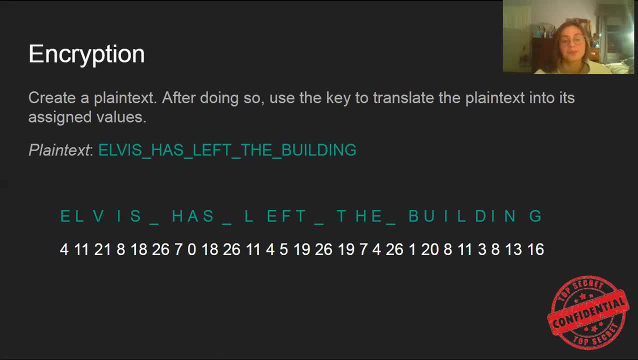 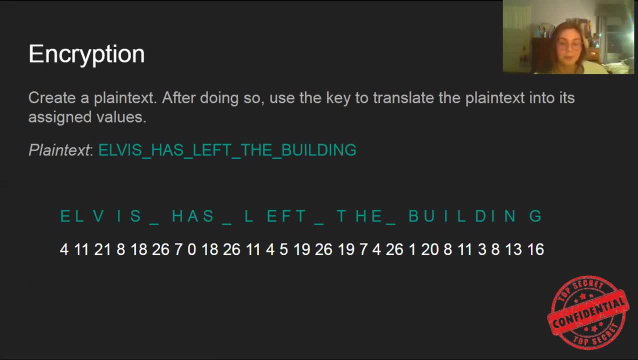 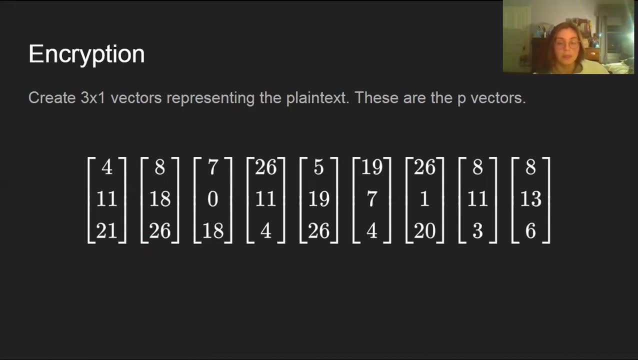 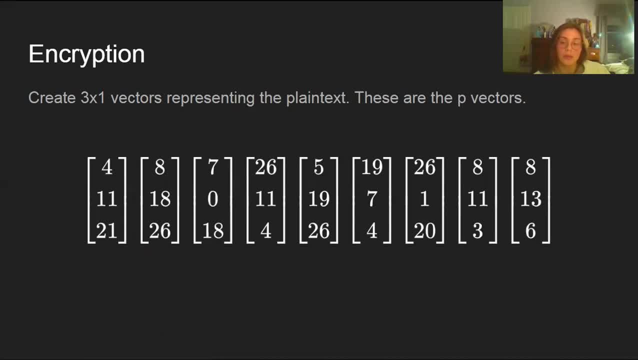 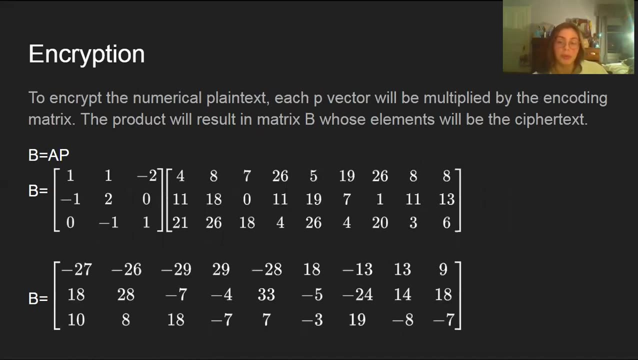 put them in 3x1 vectors because our encoding and decoding matrices are 3x3.. If these were 2x2 matrices, we'd then do 2x1 vectors And these will give us our p-vectors. Now, to encrypt the numerical plain text, each p-vector will be multiplied by the encoding. 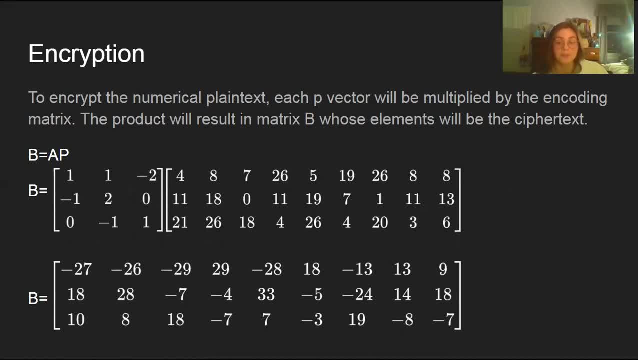 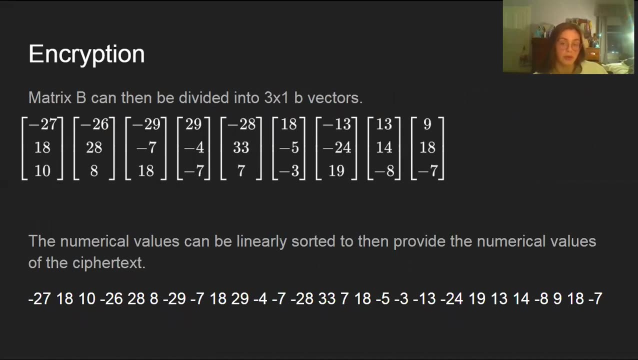 this will then give us the matrix B and these are the elements in the ciphertext. So below is just the math doing that and you can see our matrix B. and now we take matrix B and divide it into three by one vectors, we'll call B, and then once again, 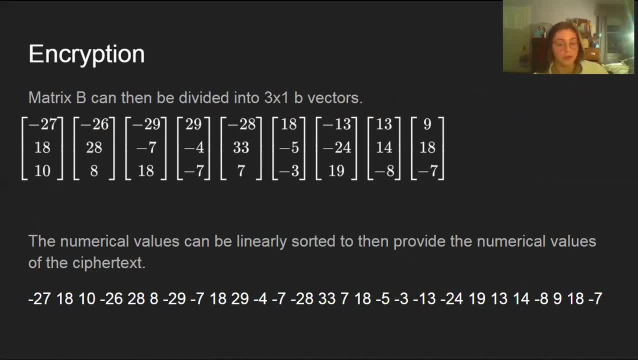 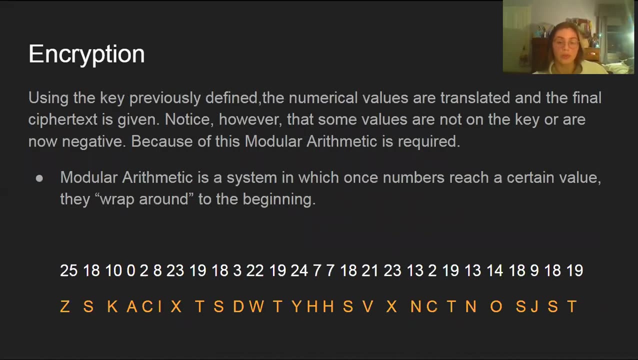 we'll take the numeric, numerical values and linearly sort them and we get the sequence of ciphertext And, as you can see, some numbers are negative, some are greater than what the key allows, and this means we'll have to use modular arithmetic. Modular arithmetic is a system in which, once numbers reach a 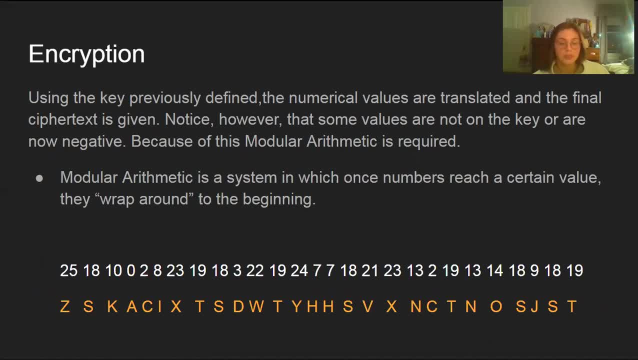 certain value. they'll wrap around to the beginning For our purposes. I'm not going to go too much into it, but here I have the modular arithmetic below, and then I assigned number to the key. So with that it gave us this encrypted message that doesn't. 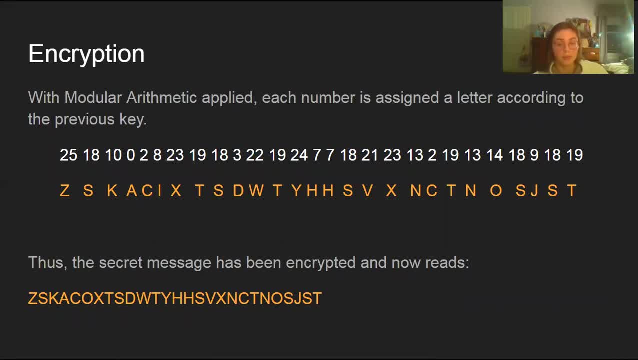 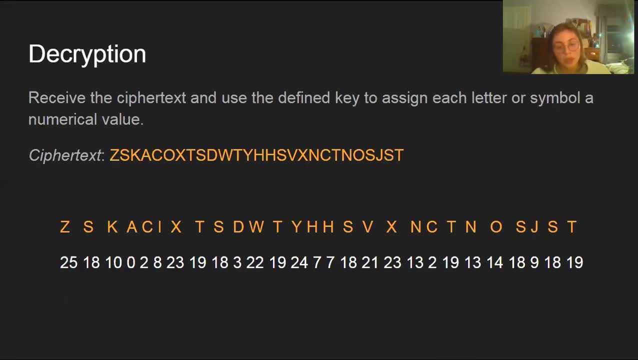 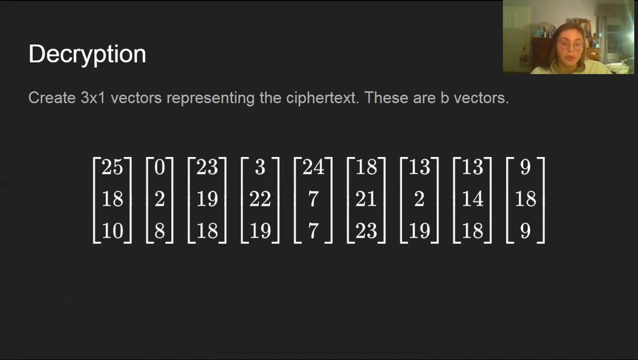 make any sense. so if a third party were to intercept it, they wouldn't know what it meant unless they had the key and the decoding matrix. Now let's decrypt this message so you'd receive the ciphertext, and once again, you use the key and assign each letter symbol to its numerical value, and then you put this: 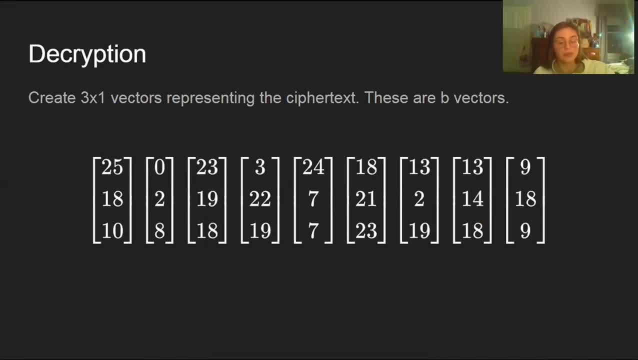 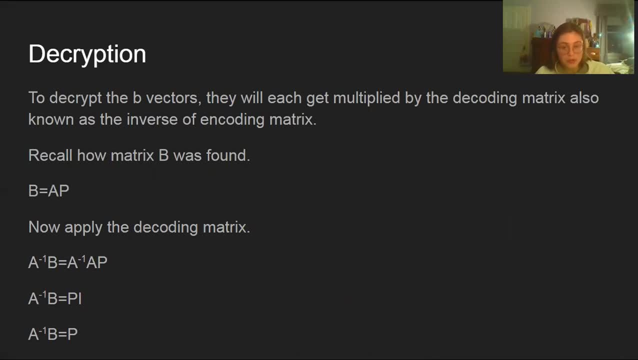 ciphertext in 3x1 vectors and these will be our V vectors. and to decrypt the B vectors, that they will get multiplied by the decoding matrix and this is the inverse of the encoding matrix. and if you look at how B was found, we multiplied the encoding matrix by our p vectors. 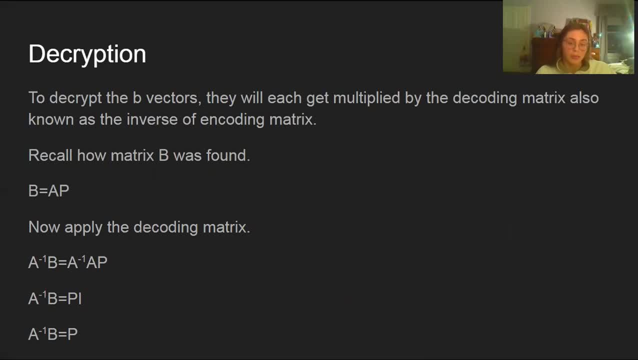 and now we are multiplying our B matrix by the decoding or inverse. So when we do that, we end up canceling the matrices- the encoding and decoding matrices on the right side, and we will end up with our P matrix back. And this is just the. 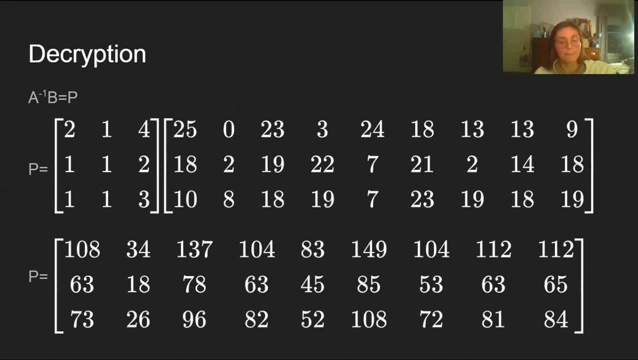 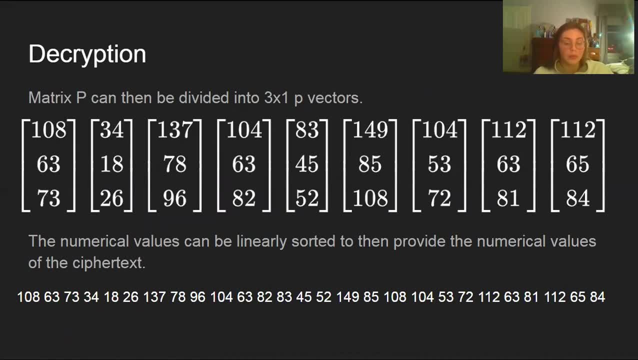 math involving that, And below is our P matrix. So the matrix P will be divided into 3 by 1 P vectors and once again these values will be linearly sorted, And below you can see that these numbers are really, really big.